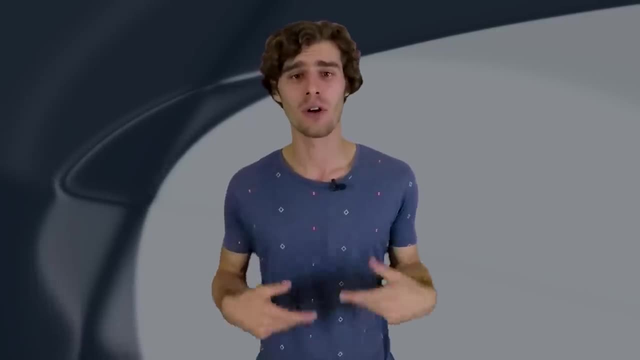 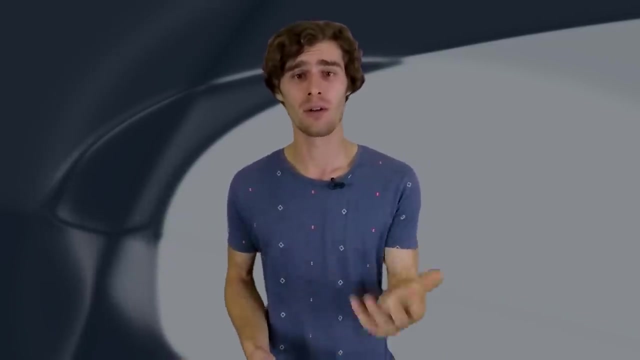 case in supervised learning, And so this means that the data distributions of our observations and rewards are constantly changing as our agent learns, which is a major cause of instability in the whole training process. And, apart from having this problem with the training data set, we also 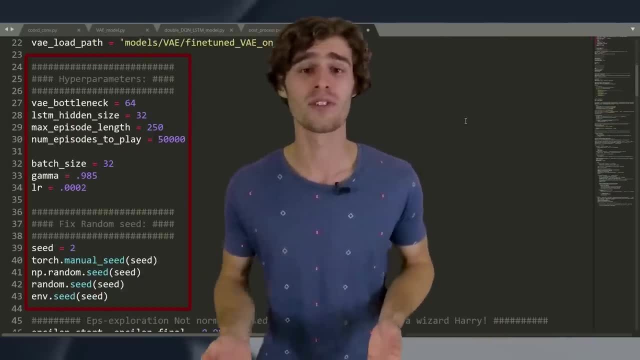 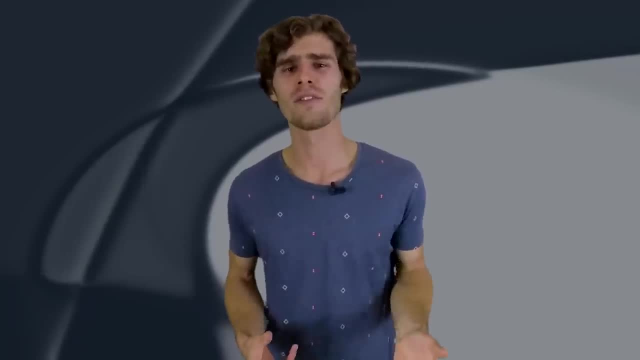 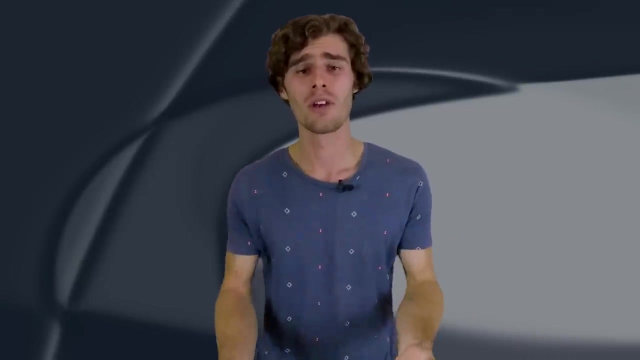 have a very high sensitivity to hyperparameter tuning and things like initialization, for example, And in some cases it's kind of intuitive to understand why this happens, because imagine that your learning rate is too large. well then, you could have a policy update that pushes your policy. 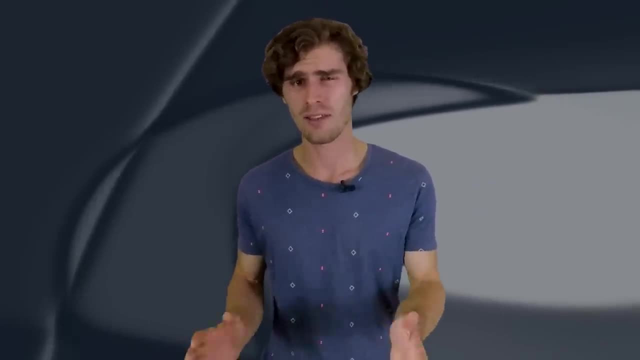 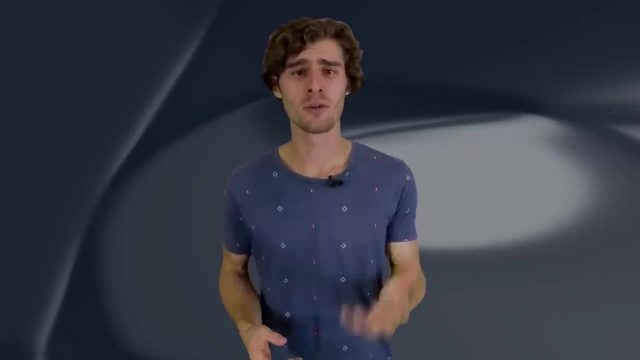 network into a region of the parameter space where it's going to collect the next batch of data under a very poor policy, causing it to never recover again. And so, to address many of these annoying reinforcement learning, the team at OpenAI designed a new reinforcement learning algorithm. 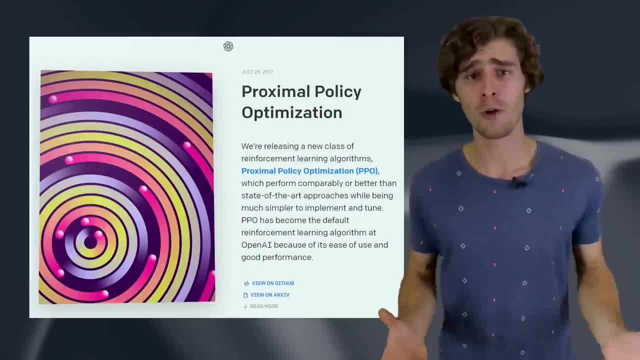 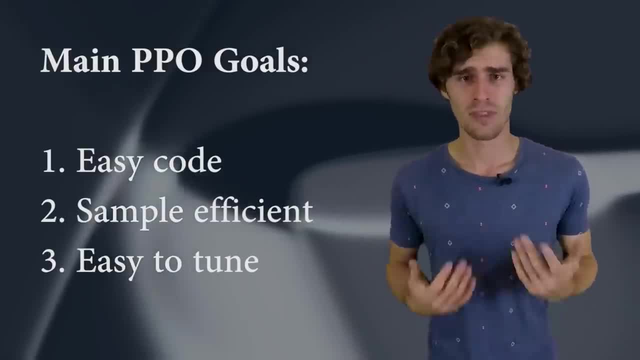 that's called Proximal Policy Optimization, or PPO, And the core purpose behind PPO was to strike a balance between ease of implementation, sample efficiency and ease of tuning. Now, the first thing to realize about PPO is that it is what we call a policy gradient method, And this means that 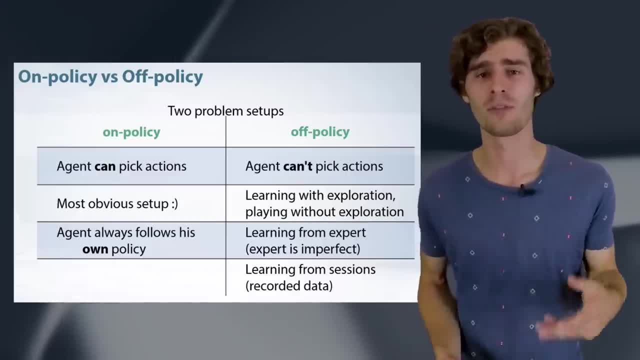 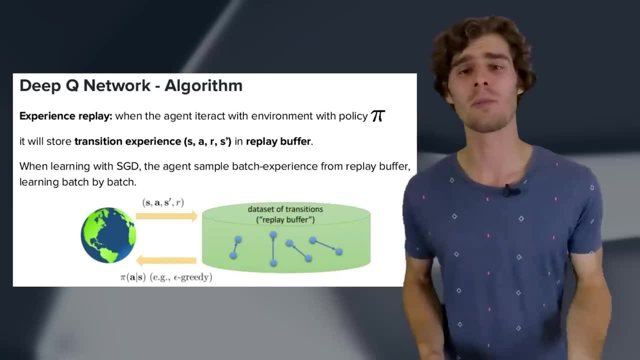 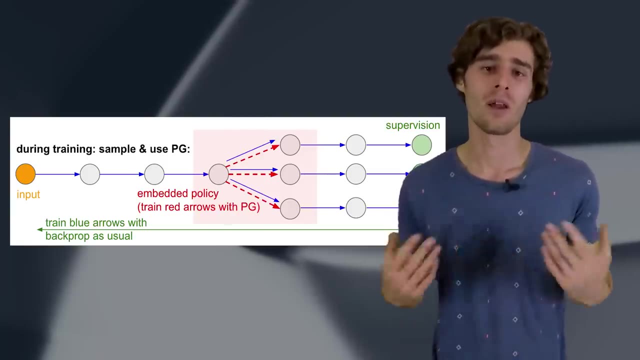 unlike popular Q-learning approaches like DQN, for example, that can learn from stored offline data, Proximal Policy Optimization learns online And this means that it doesn't use a replay buffer to store past experiences, but instead it learns directly from whatever its agent encounters in the environment. 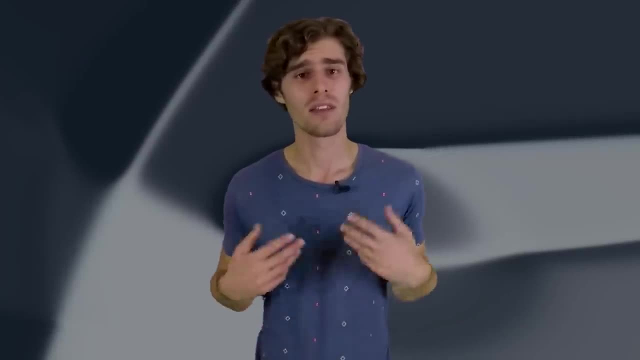 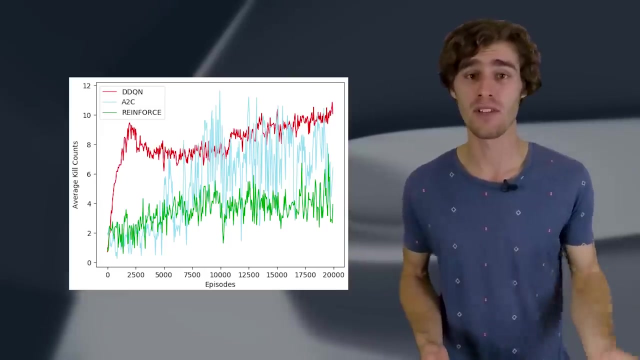 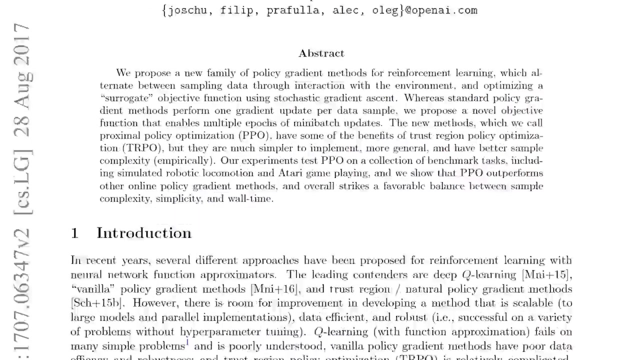 And once a batch of experience has been used to do a gradient update, the experience is then discarded and the policy moves on. And this also means that policy gradient methods are typically less sample efficient than Q-learning methods, because they only use the collected experience once for doing an update And now general policy optimization methods usually start by defining the 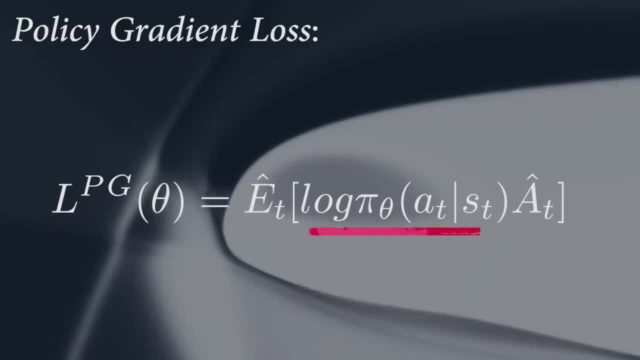 policy gradient laws that are associated with a Columbia Eполy And to look at the policy optimization methods can be as follows: that are associated with a Columbia Epoly And to look at the policy optimization methods can be as follows: as the expectation over the log of the policy actions times an estimate of the advantage, 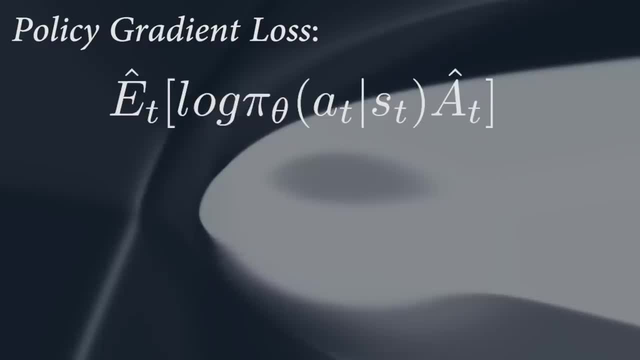 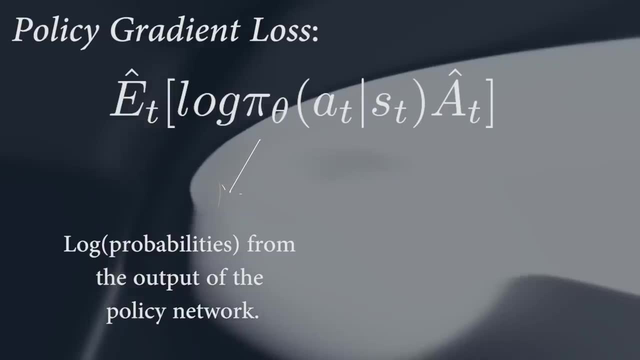 function Okay. so what does that all mean? Well, the first term, pi theta, is our policy. It's a neural network that takes the observed states from the environment as an input and suggests actions to take as an output. And the second term is the advantage function a, which basically tries. 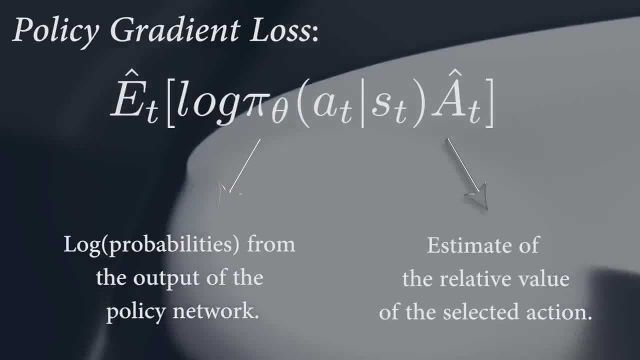 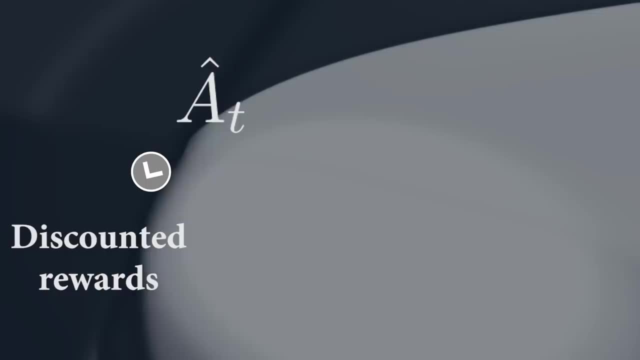 to estimate what the relative value is of the selected action in the current state. So let's take apart what that means. So, in order to compute the advantage, we need two things: We need the discounted sum of rewards and we need a baseline estimate. And so the first part is the discounted 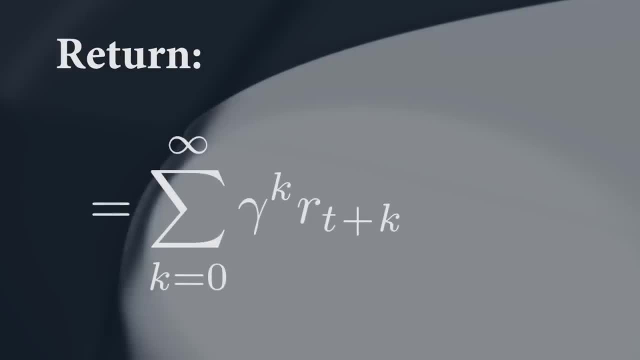 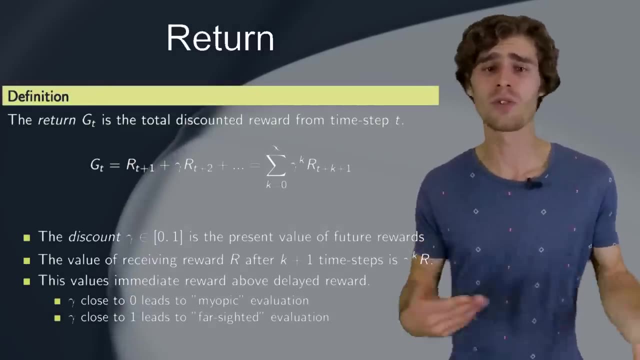 sum of rewards or the return, And this is basically a weighted sum of all the rewards the agent got during each time step in the current episode. And then the discount factor gamma, which is usually somewhere between 0.9 and 0.99, accounts for the fact that your agent cares more about reward that. 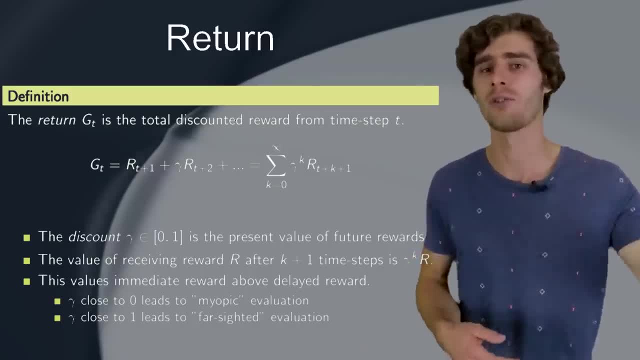 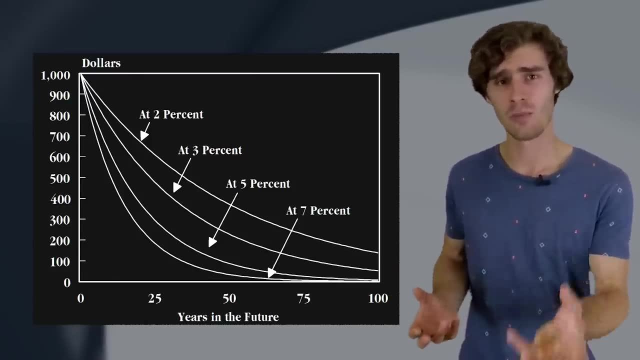 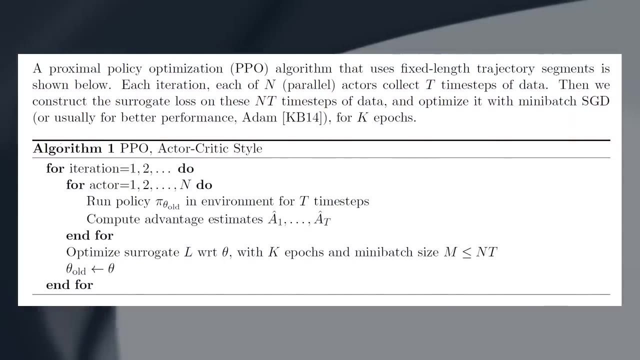 is going to get very quickly. versus the same reward, It would get 100 time steps for now, And this is exactly the same idea as interest in the financial world, in the sense that getting money tomorrow is usually more valuable than getting the same amount of money, say, a year from now, And so notice that the advantage is calculated after. 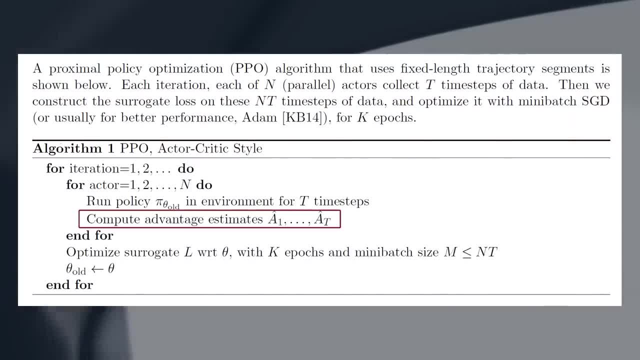 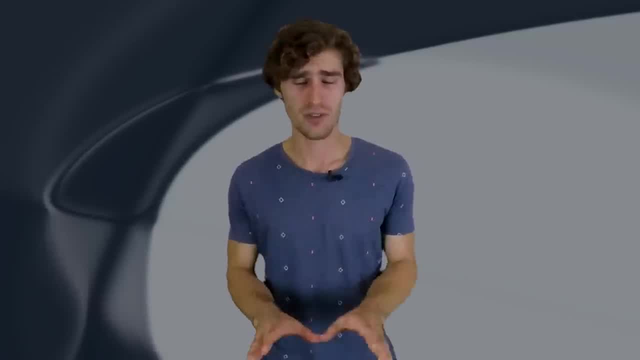 the episode sequence was collected from the environment. So, in other words, we know all the rewards, So there is no guessing involved in computing the discounted return, because we actually know what happened. Okay, so that was the first part of the advantage function. 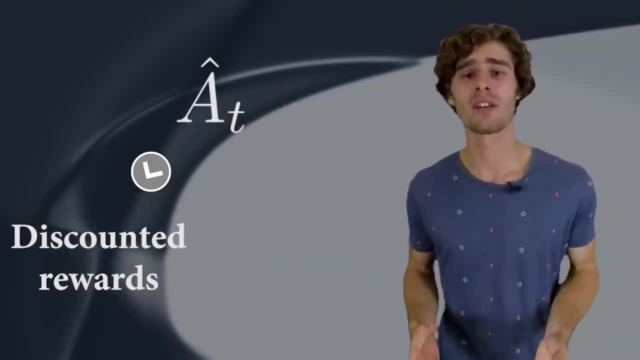 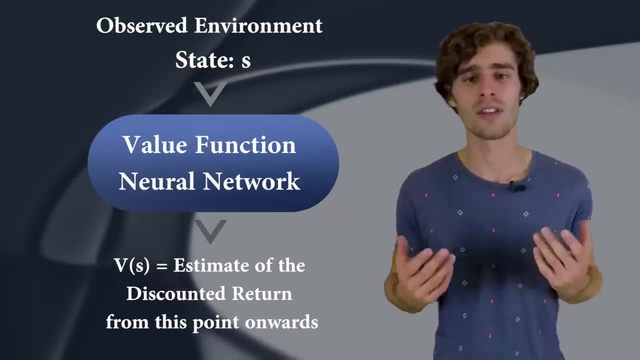 the discounted sum of rewards, And then the second part of the advantage function is the baseline or the value function, And basically what the value function tries to do is give an estimate of the discounted sum of rewards from this point onwards. So basically it's trying to guess what the final return is going to be in. 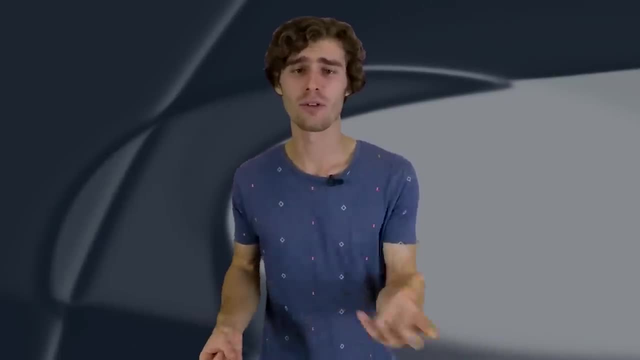 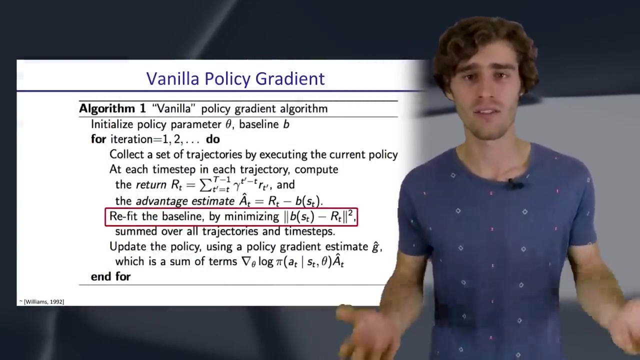 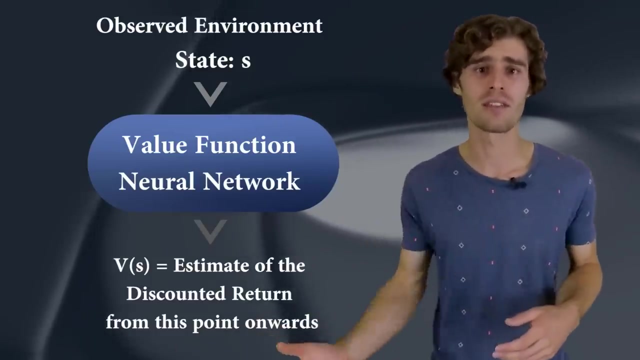 this episode starting from the current state And during training. this neural net that's representing the value function is going to be frequently updated using the experience that our agent collects in the environment, because this is basically a supervised learning problem. You're going to use the states as an input and your neural net is trying to predict what the discounted sum of 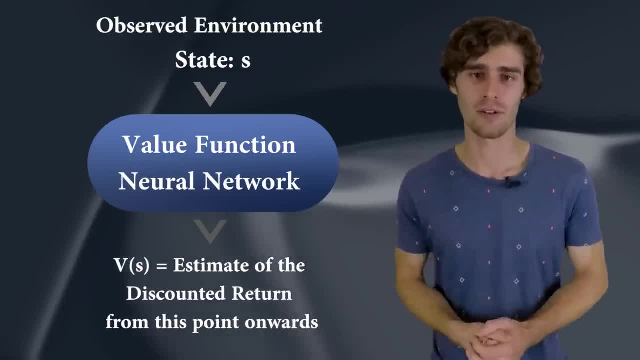 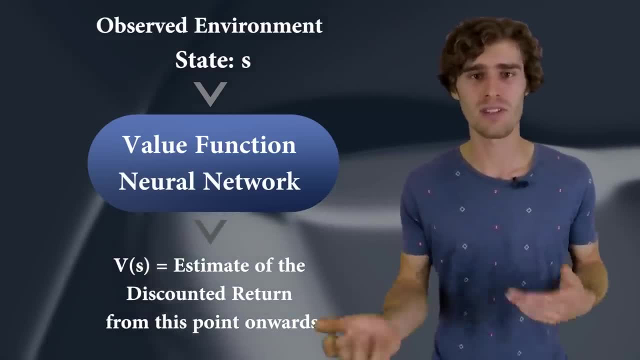 rewards is going to be from this state onwards. So basic supervised learning. And notice that, because this value estimate is the output of a neural net, this is going to be a noisy estimate. There's going to be some variance because our network is not going to always predict the exact value of that. 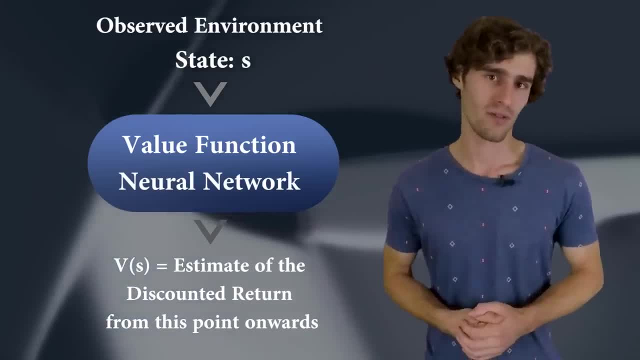 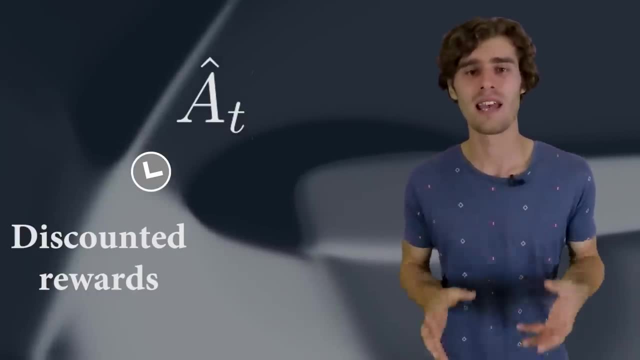 state. So, basically, we're going to end up with a noisy estimate of the value function. Okay. so now we have the two terms that we need, We have the discounted sum of rewards that we computed from the result rollout and we have an expectation, an estimate of that value, given the state that. 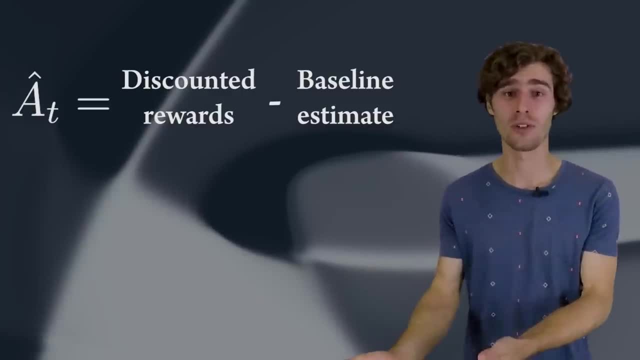 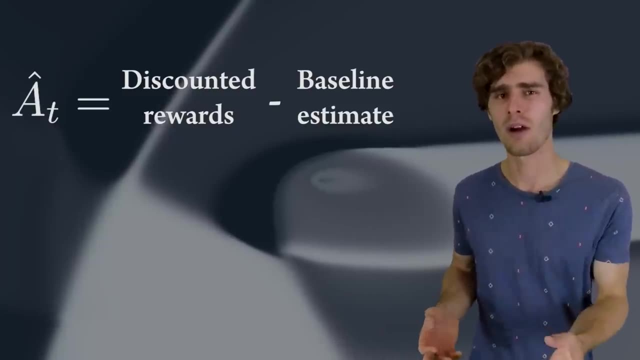 we're in, And if we then subtract the baseline estimate from the actual return we got, we get what we call the advantage estimate. And so, basically, the advantage estimate is answering the question: how much better was the action that I took, based on the expectation of what would 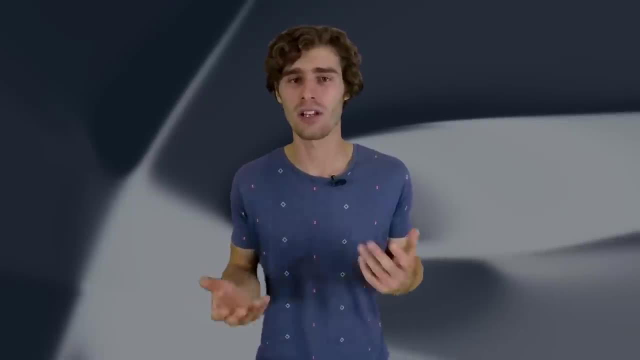 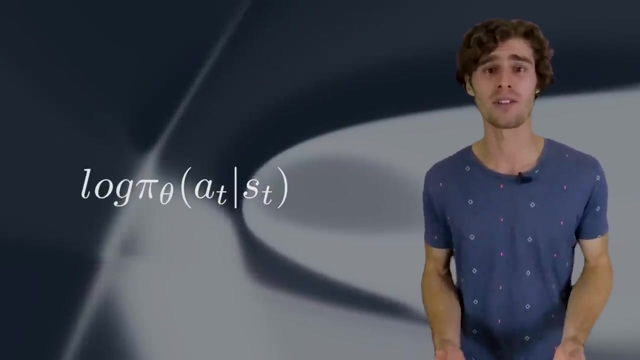 normally happen in the state that I was in. So, basically, was the action that our agent took? was it better than expected or was it worse? And so then, by multiplying the log probabilities of your policy actions with this advantage function, we get the final optimization. 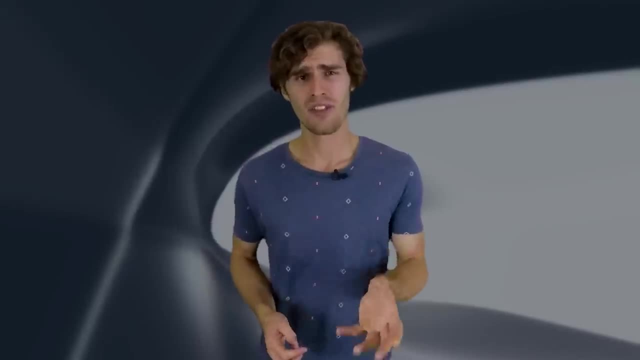 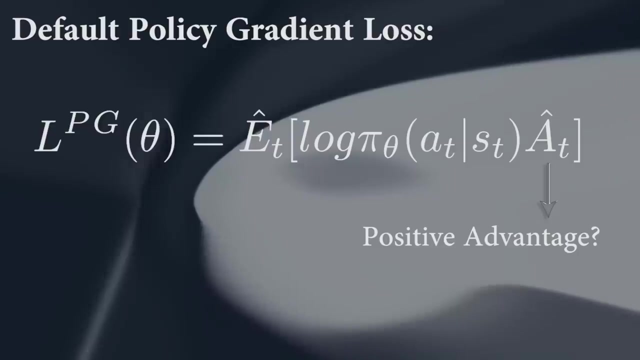 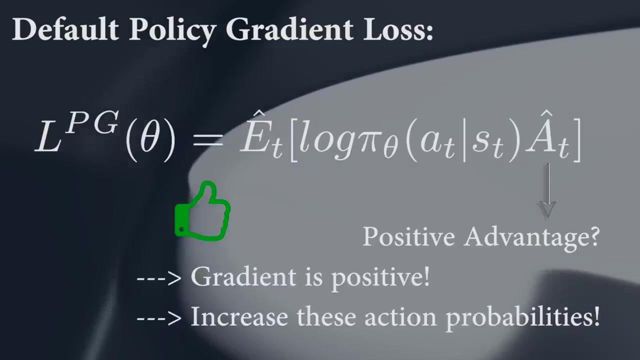 objective that is used in policy gradient And if you think about what this objective function is doing, it's intuitively satisfying because if the advantage estimate was positive, meaning that the actions that the agent took in the sample trajectory resulted in better than average return, what we'll do is we'll increase the probability of selecting them again in the 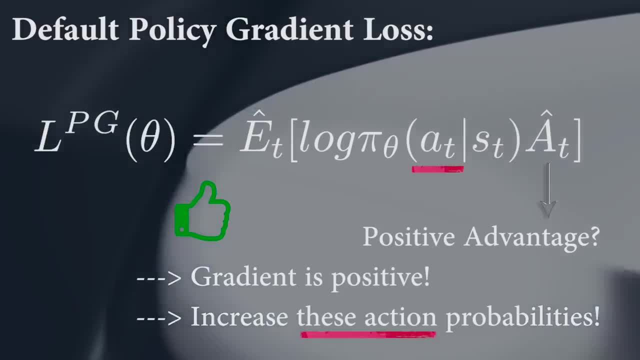 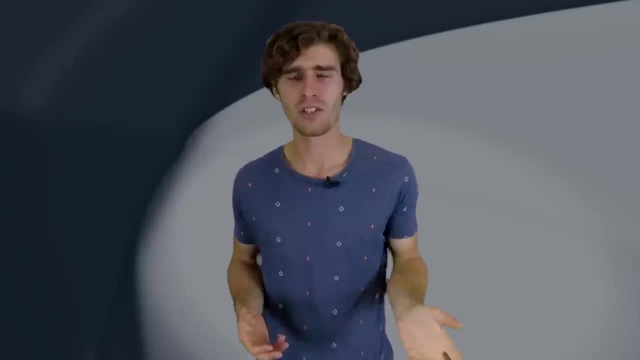 future, when we encounter the same state, And if, on the other hand, the advantage function was negative, then we'll reduce the likelihood of the selected actions, which makes total sense. right And now, as I've already mentioned, one of the problems is that if you simply keep running, 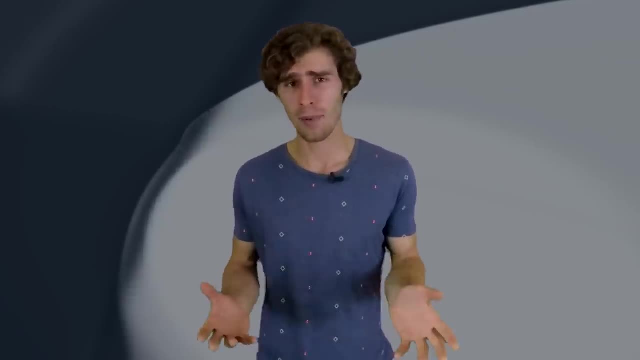 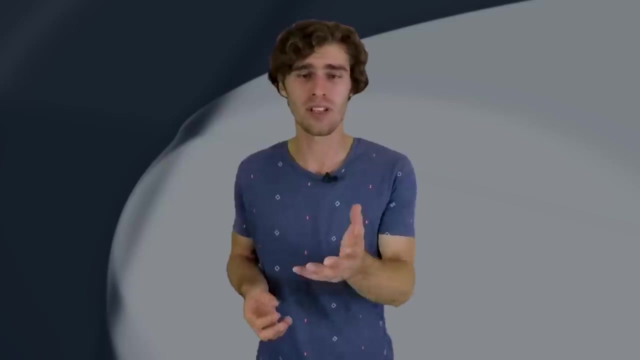 gradient descent on one batch of collected experience. what will happen is that you'll update the parameters in your network so far outside of the range where this data was collected. that, for example, the advantage function, which is, in principle, a noisy estimate of the real 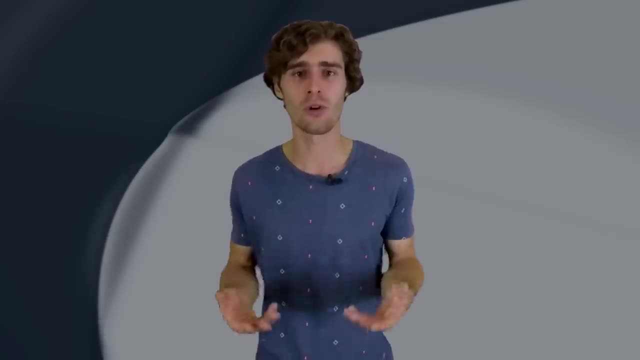 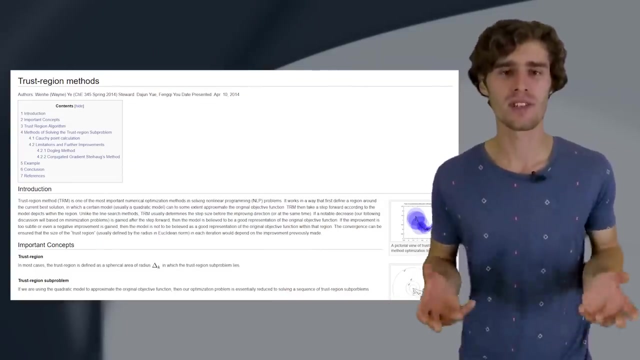 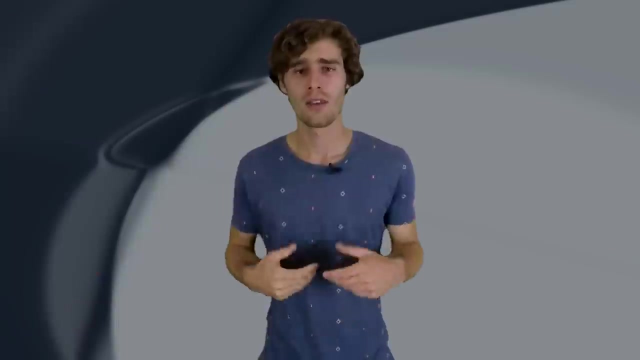 advantage is going to be completely wrong, And so, in a sense, you're just going to destroy your policy if you keep running gradient descent. And now to solve this issue, one successful approach is to make sure that, if you're updating the policy, you're never going to move too far away from the old policy. Now, this idea was widely 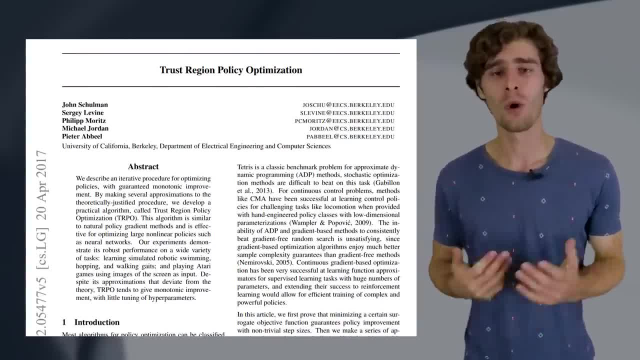 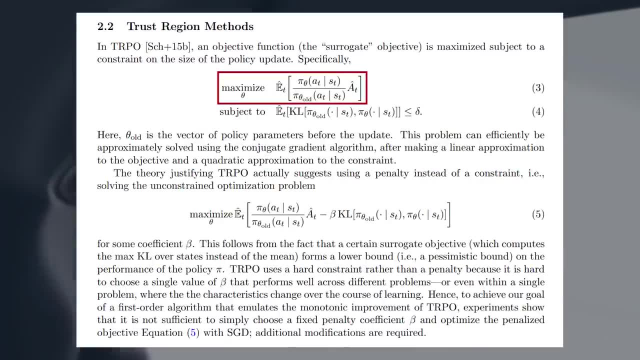 introduced in a paper called Trust Region Policy Optimization, or TRPO, which is actually the whole basis on which PPO was built. And so here is the objective function that was used in TRPO And, if you compare this with the previous objective function for vanilla policy gradients, what you 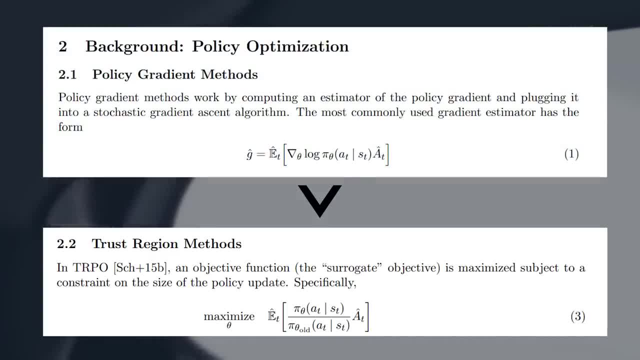 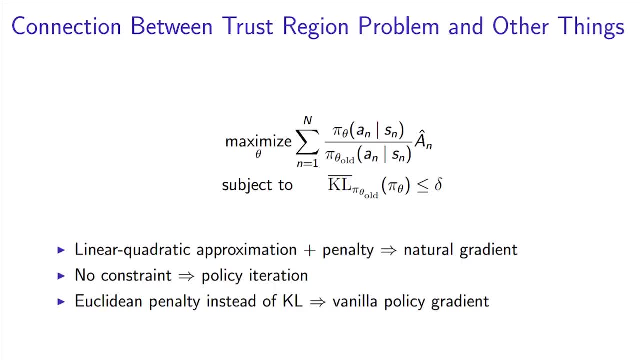 can see is that the only thing that TRPO was able to do in the previous objective function was to replace the log operator with a division by pi-theta-old. Now the slide here shows that optimizing this TRPO objective is in fact identical to vanilla policy gradients. I'm not going to go. 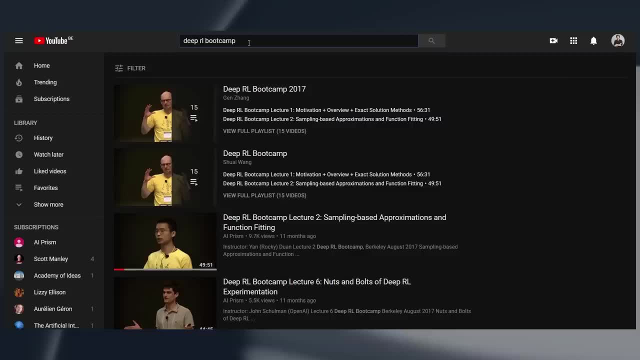 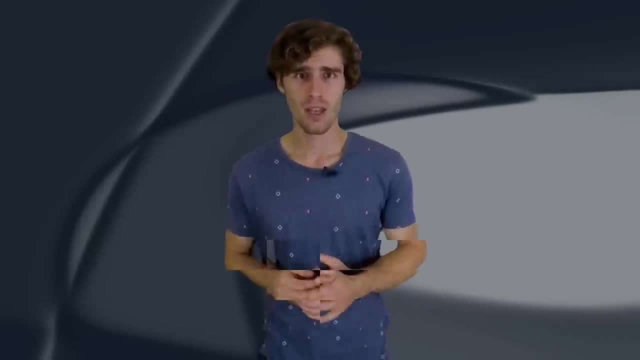 into the derivation details here, but if you want, you can pause the video or check out lecture 5 of the DeepRL Bootcamp, which will take you deep down the rabbit hole Link in the description. Now to make sure that the updated policy doesn't move too far away from the current policy. 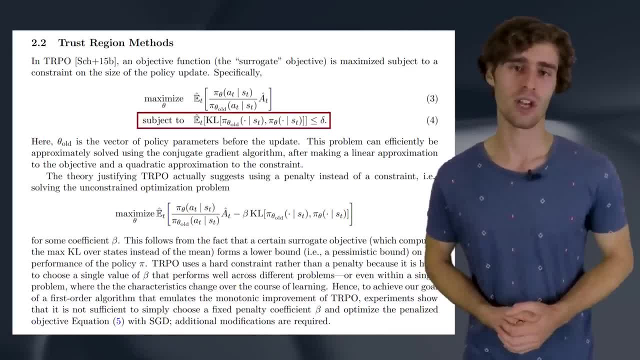 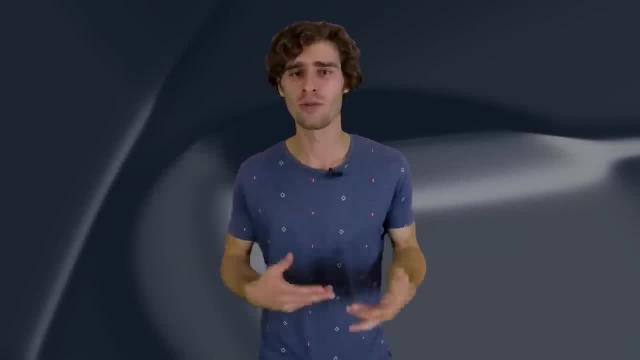 TRPO adds a k-added policy to the old policy, And so in this case, you can see that the k-added policy is not moved too far away from the old policy, And so what this k-al constrained effectively does is it's just going to make sure that the new updated policy doesn't move too far. 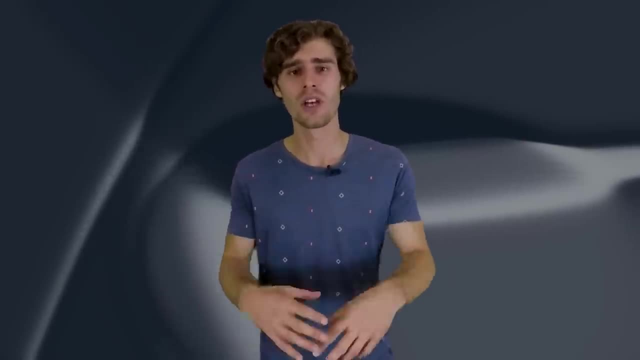 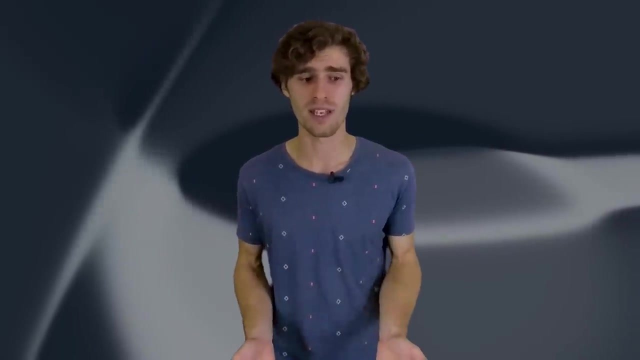 away from the old policy. So in a sense we just want to stick close to the region where we know everything works fine. The problem is that this k-al constrained adds additional overhead to our optimization process and can sometimes lead to very undesirable training behavior. So 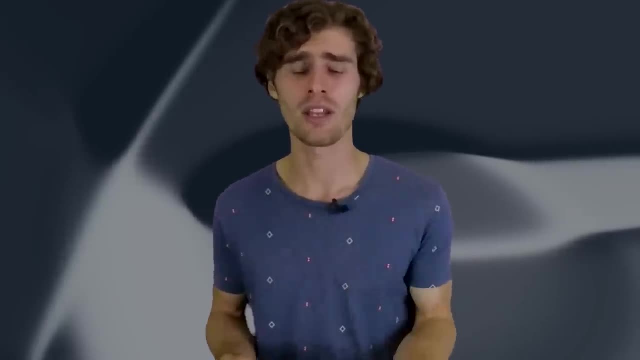 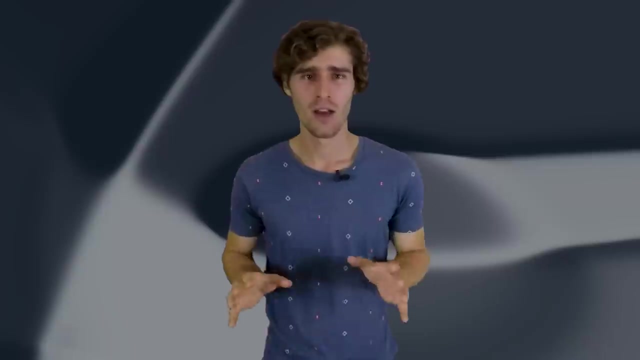 wouldn't it be nice if we can somehow include this extra constraint directly into our optimization objective? Well, as you might have guessed, that is exactly what PPO does. Okay, so now that we have a little bit of surroundings, let's dive into the crux of the algorithm. the central 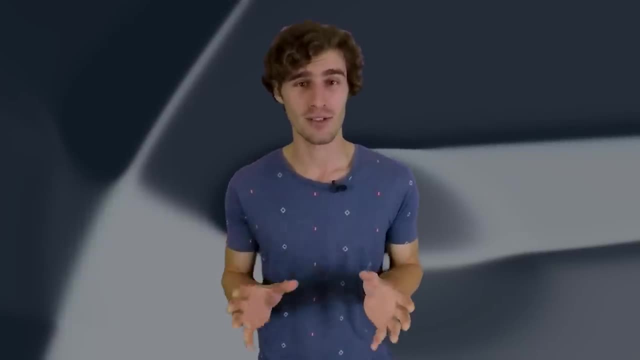 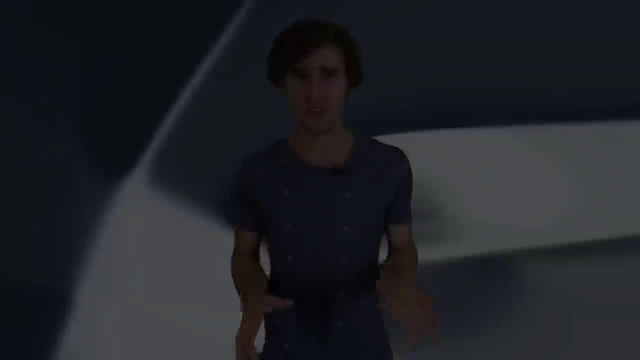 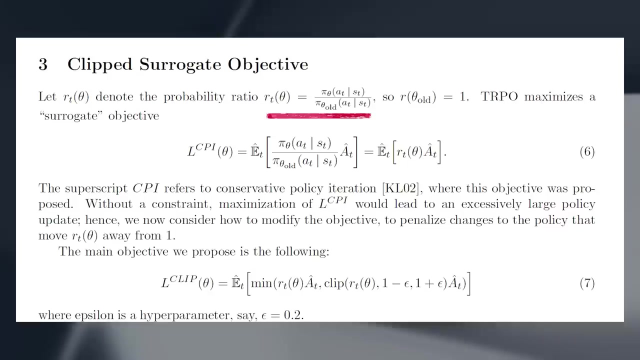 optimization objective behind PPO. Hold on to your hats, it's about to get a little technical. So first let's define a variable, r theta, which is just the probability ratio between the new, updated policy outputs and the outputs of the previous, old version of the policy network. 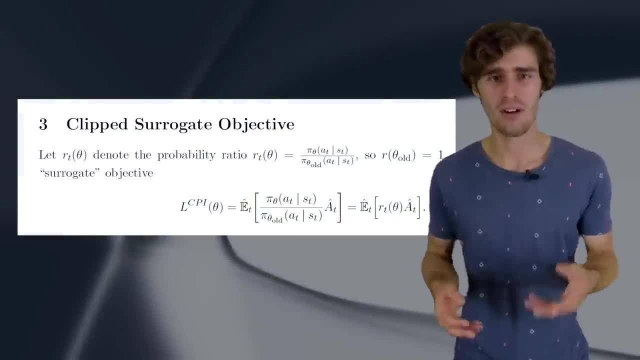 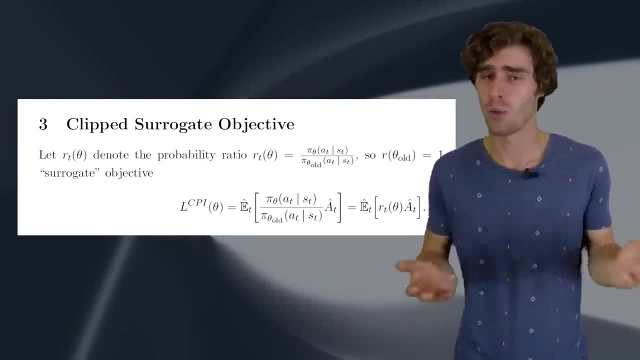 So, given a sequence of sampled actions and states, this r theta value will be larger than one if the action is more likely now than it was in the old version of the policy, And it will be somewhere between zero and one if the action is less likely now than it was before the last gradient step. 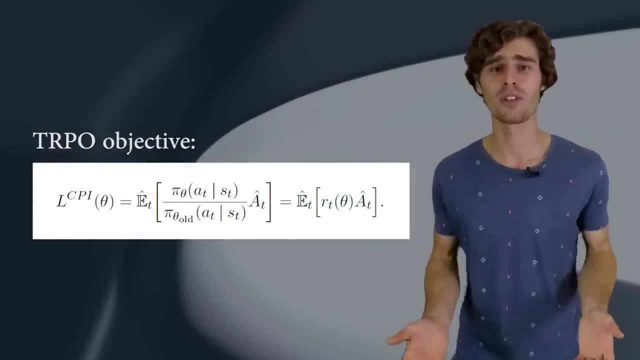 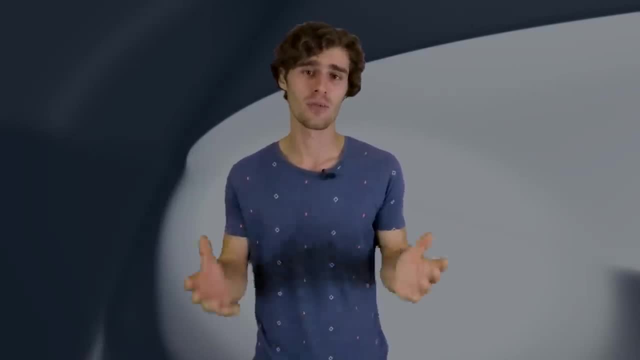 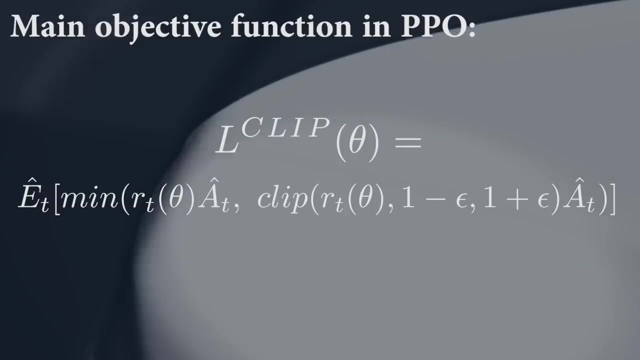 And then, if we multiply this ratio r- theta with the advantage function, we get the normal TRPO objective in a more readable form, And with this notation we can finally write down the central objective function that is used in PPO. Here it is Looks surprisingly simple, right? Well, first of all, you can see that the objective 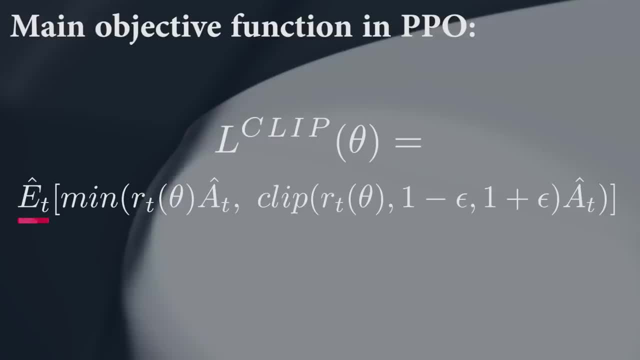 function that PPO optimizes is an expectation operator. So this means that we're going to compute this over batches of trajectories And this expectation operator is taken over the minimum of two terms. The first of these terms is r? theta times the advantage estimate. So this is the 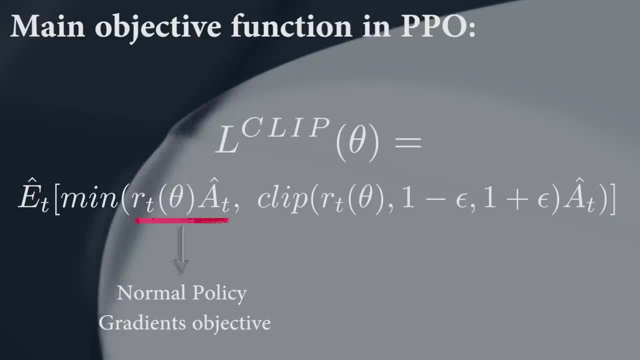 default objective for normal policy gradients, which pushes the policy towards actions that yield positive advantage over the baseline. Now, the second term is very similar to the first one, except that it contains a truncated version of this r? theta ratio by applying a clipping operation between: 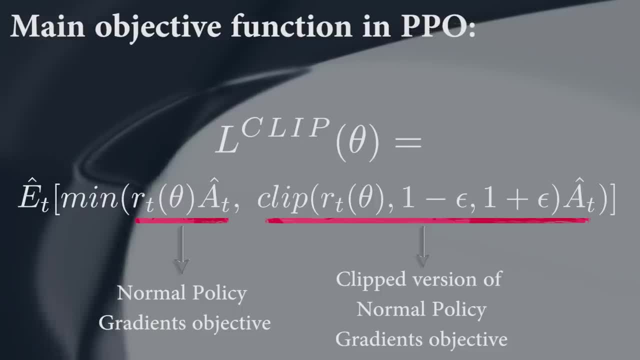 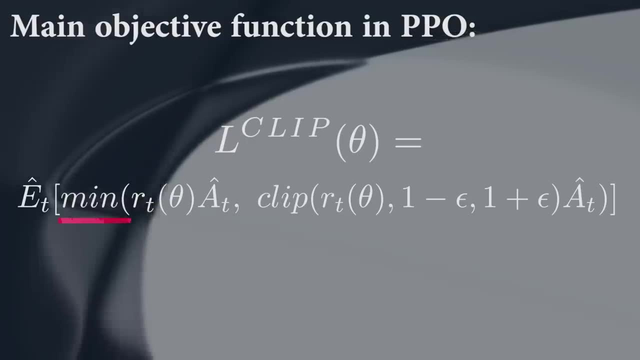 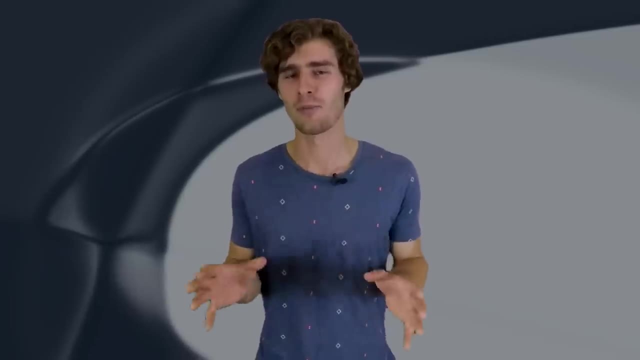 one minus epsilon and one plus epsilon, where epsilon is usually something like 0.2.. And then, lastly, the min operator is applied to the two terms to get the final result. And while this function looks rather simple at first sight, fully appreciating all the subtleties of work here takes a little bit. 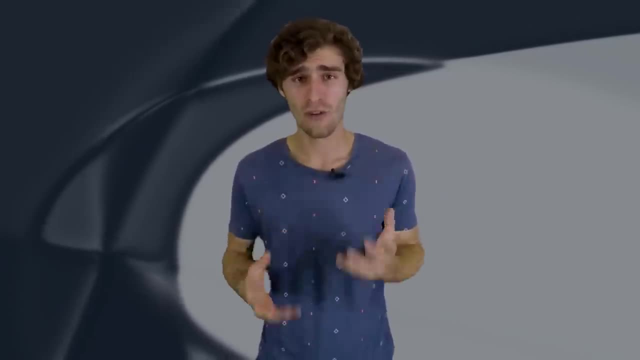 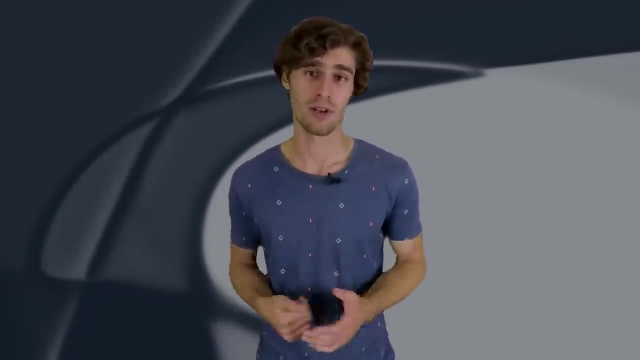 more effort. Bear with me here. I promise we're almost there. Firstly, it's important to note that the advantage estimate can be both positive and negative, and this changes the effect of the min operator. Here is a plot of the objective function for both positive and negative values. 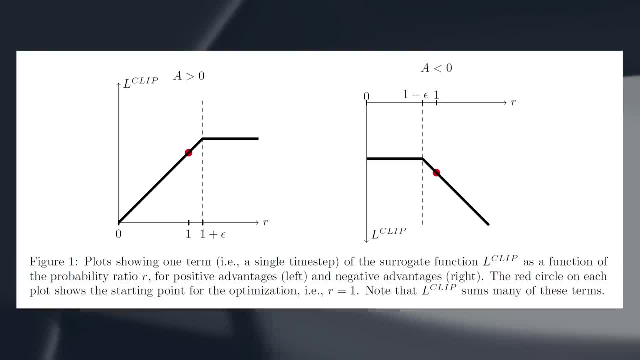 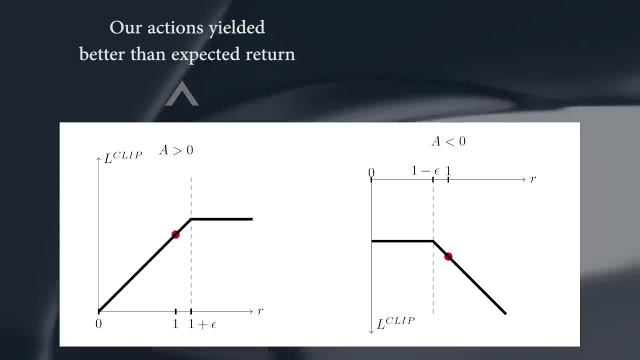 of the advantage estimate. So on the left half of the diagram, where the advantage function is positive, are all the cases where the selected action had a better-than-expected effect on the outcome, And on the right half of the diagram we can find situations where the action 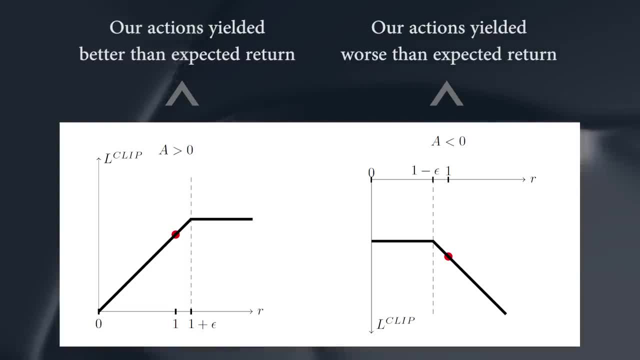 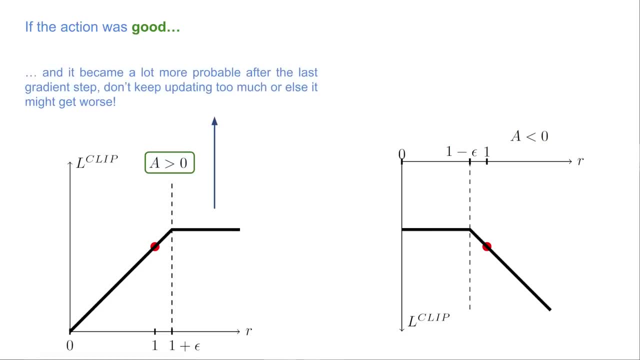 had an estimated negative effect on the outcome. Now, on the left side, notice how the loss function flattens out when r gets too high. And this happens when the action is a lot more likely under the current policy than it was under the old policy, And in this case we don't want to overdo the action. 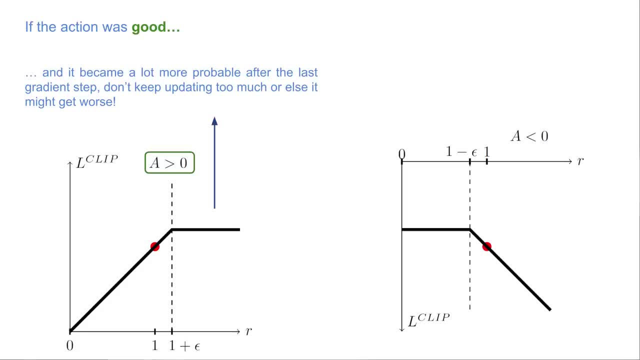 update too much, and so the objective function gets clipped here to limit the effect of the gradient update. And then, on the right side, where the action had an estimated negative value, the objective function flattens out when r goes near zero, And this corresponds to actions that are much. 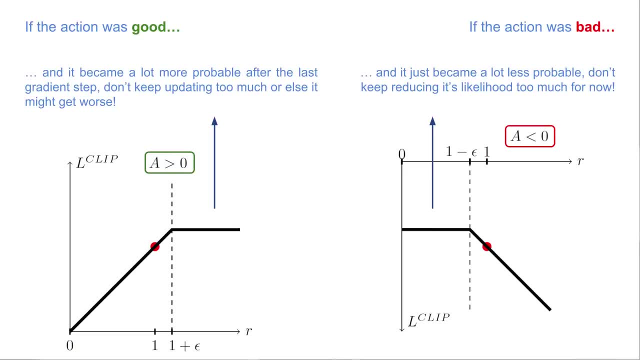 less likely now than in the old policy and we'll have the same effect of not overdoing a similar update which might otherwise reduce the action probabilities to zero. Remember the advantage: function is noisy, so we don't want to destroy a policy based on a single estimate. 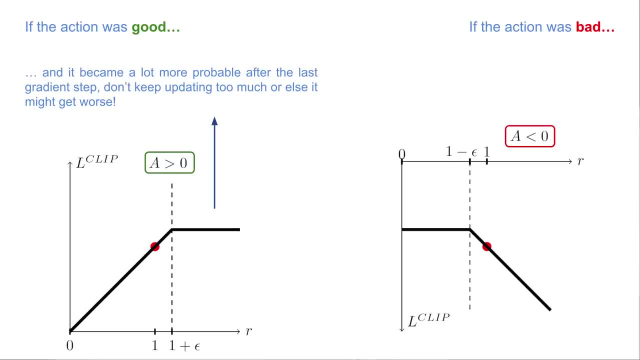 And finally, what about the very right-hand side? Well, the objective function only ends up in this region when the loss gradient step made the selected action a lot more probable. so r is big, while also making our policy worse, since the advantage is negative here. and if that's the case, 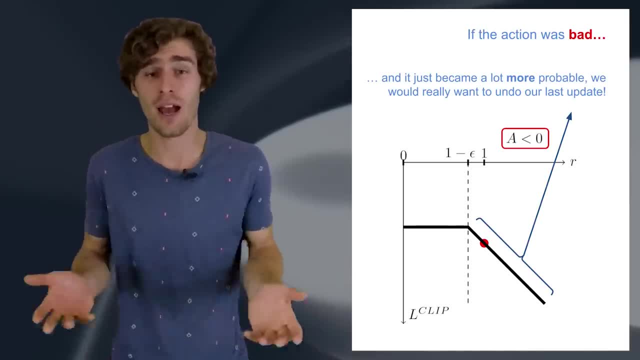 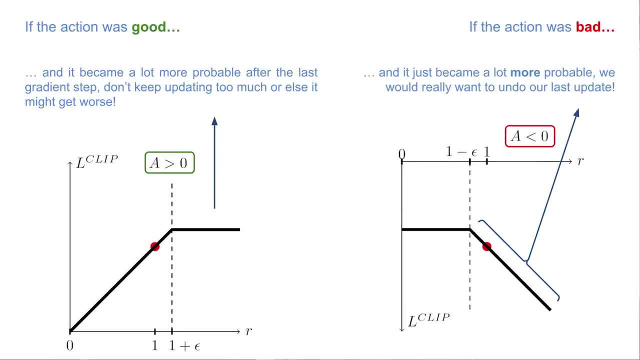 then we would really want to undo the last gradient step, and it just so happens that the objective function in ppo allows us to do this. the function is negative here, so the gradient will tell us to walk the other direction and make the action less probable by an amount proportional to how much we 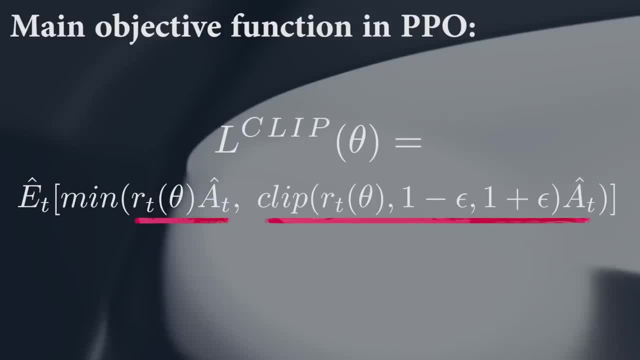 screwed it up in the first place. and also notice that this is the only region where the unclipped part of the objective function has a lower value than the clipped version and thus gets returned by the minimization operator. pretty clever, right? and if you're wondering how on earth the authors 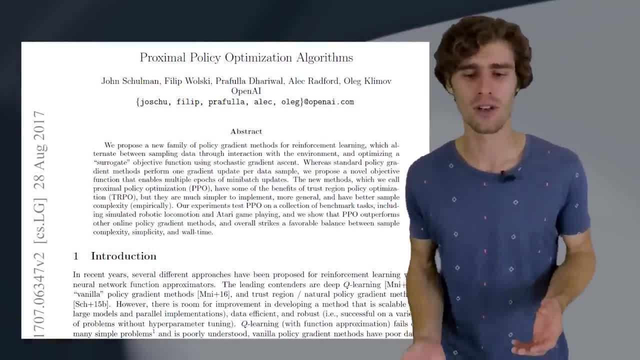 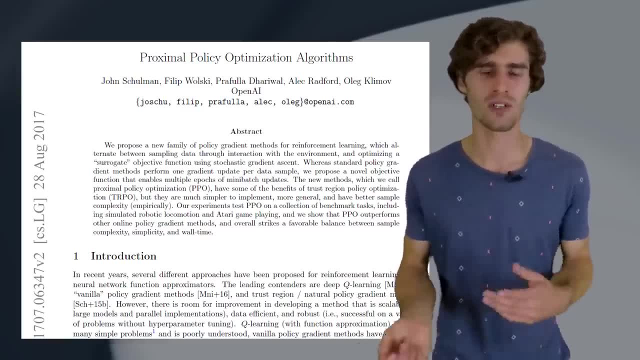 from the ppo paper managed to design this specific reward function well. it's quite likely that they had an intuitive idea of what they wanted the objective function to do, so they probably sketched a bunch of diagrams that satisfied the behavior that we just discussed and then came up with the 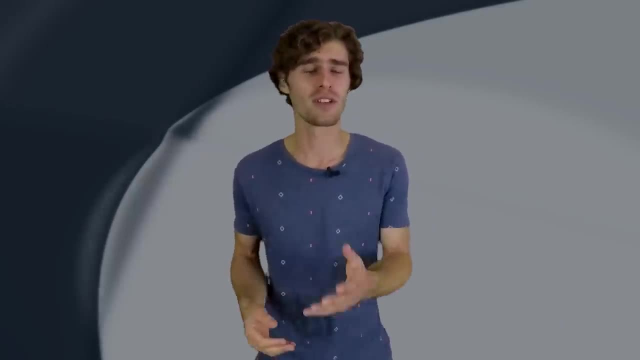 exact objective function to make it all work out. and don't worry about it if you don't have the objective function yet. and don't worry about it if you don't have the objective function yet. don't worry if you didn't fully get all the little details involved. basically, the ppo objectives does. 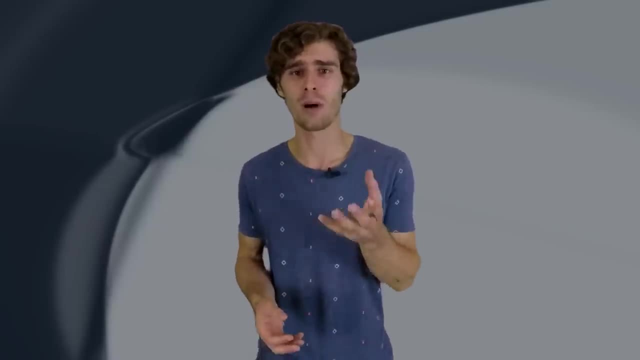 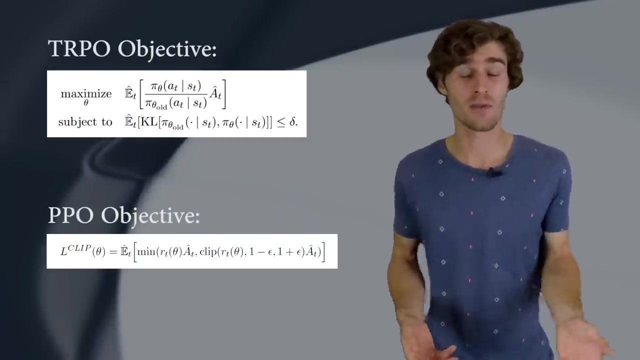 the same as the trpo objective in that it forces the policy updates to be conservative if they move very far away from the current policy. the only difference is that ppo does this with a very simple objective function that doesn't require to calculate all these additional constraints or kl. 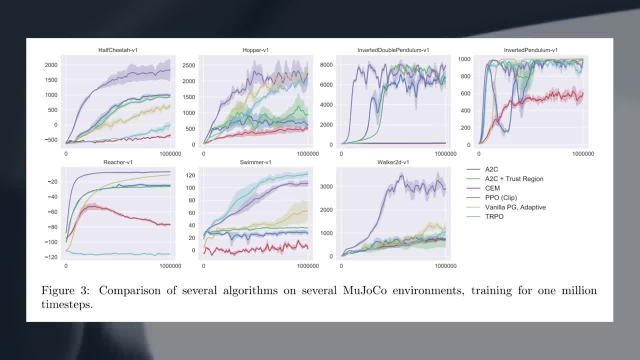 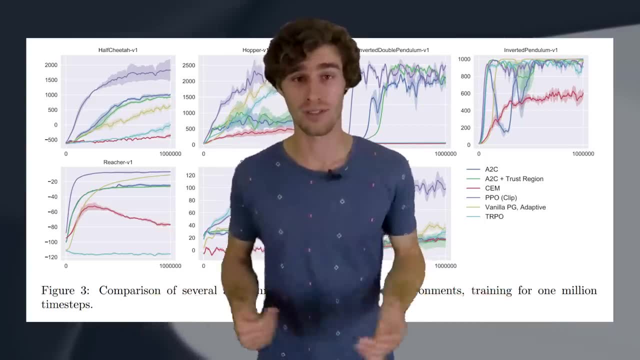 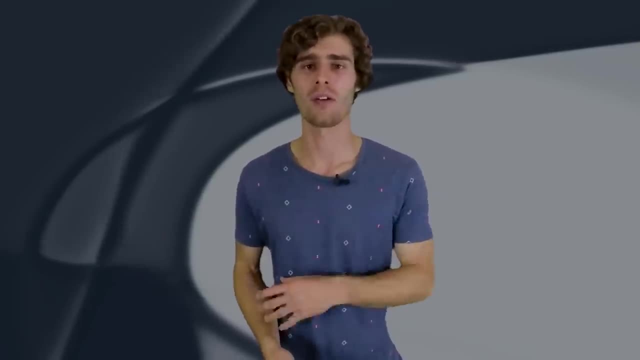 divergences and in fact, it turns out that the simple ppo objective function often outperforms the more complicated variant that we have in trpo. simplicity often wins all right, nice. now that we've seen the central objective function behind ppo, let's take a look at the entire algorithm, end to end. so, as mentioned before, there are two. 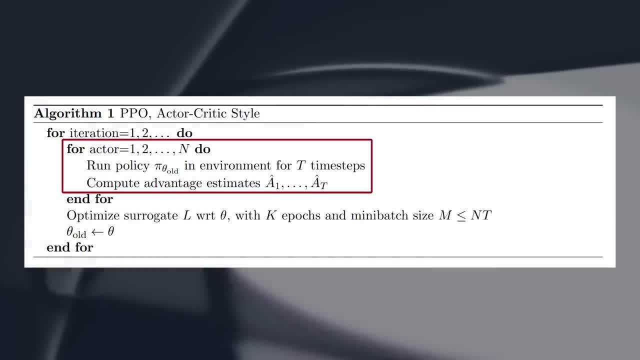 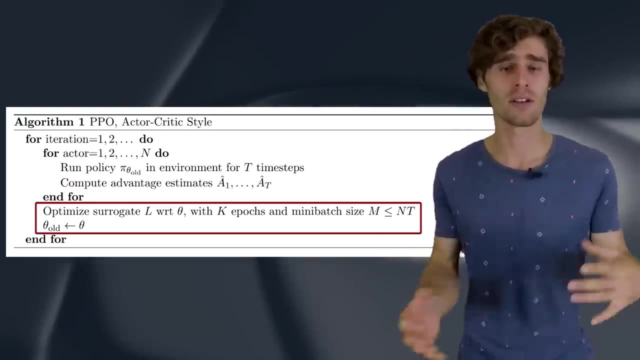 alternating threads in ppo. in the first one, the current policy is interacting with the environment, generating episode sequences for which we immediately calculate the advantage function using our fitted baseline estimate for the state values. and then, every so many episodes, a second thread is generated and the second thread is generated and the third thread is generated. 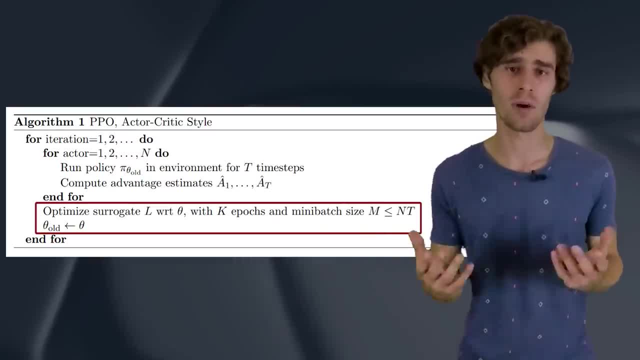 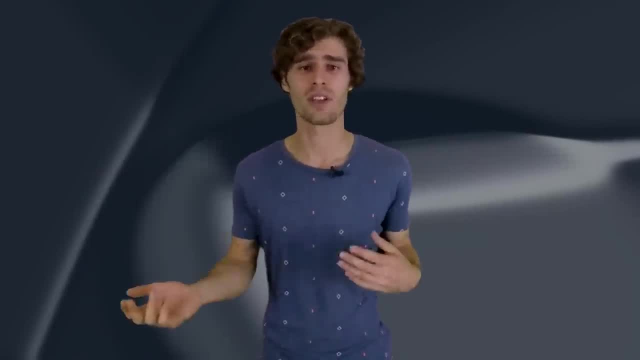 is going to collect all that experience and run gradient descent on the policy network using the clipped ppo objective and, as was done in training, the opening i5 system. these two threads can actually be decoupled from each other by using thousands of remote workers that interact with the 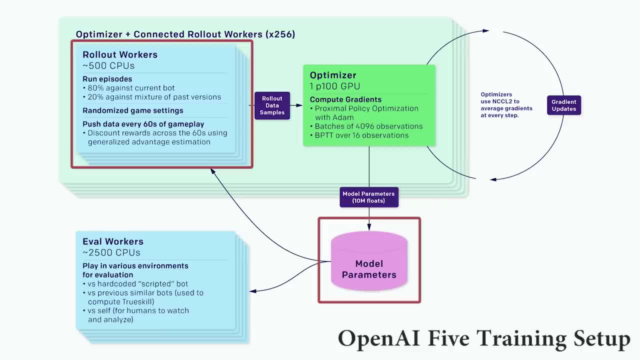 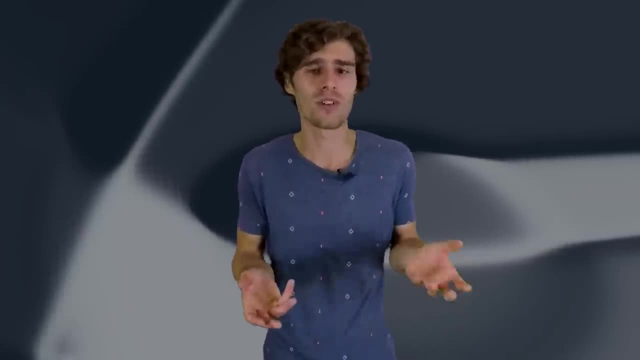 environment using a recent copy of the policy network and a gpu cluster that runs gradient descent on the network weights, using the collected experience from those workers. note that in this case each worker has to refresh its local copy of the policy network pretty often to make sure that it's always running with the latest. 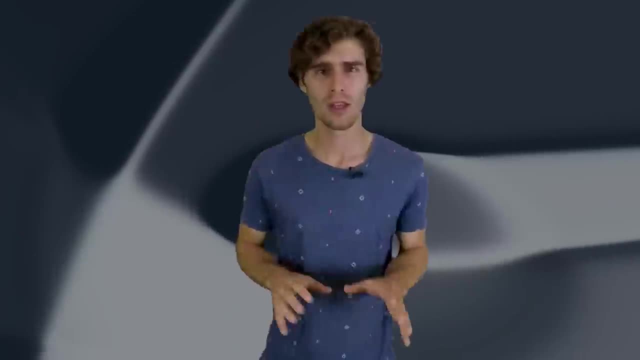 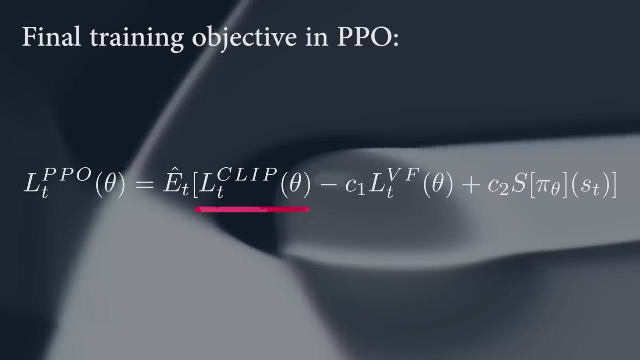 version of the policy network to keep everything nicely balanced. now, importantly, the final loss function that is used to train an agent is the sum of this clipped ppo objective that we just saw, plus two additional terms. the first additional term of the loss function is basically in charge. 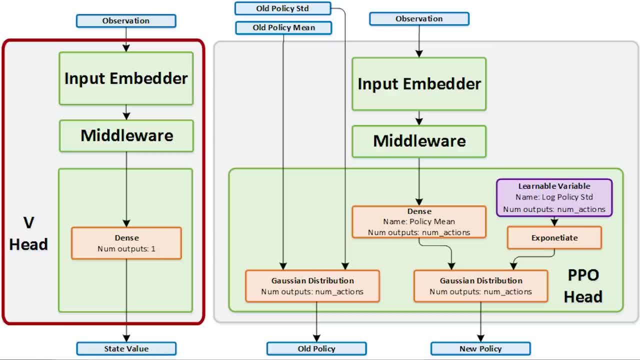 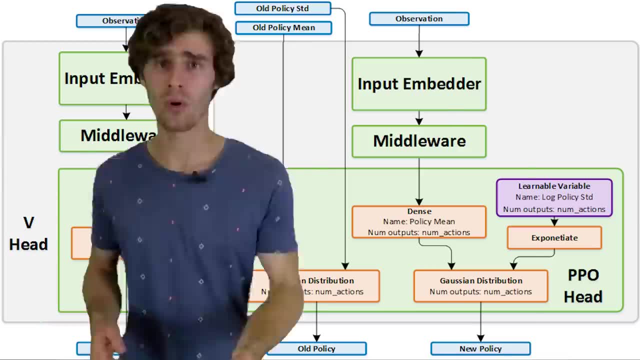 of updating the baseline network. so this is the part of the network graph that is in charge of estimating how good it is to be in this state or, more specifically, what is the average of the loss function and the average amount of discounted reward that i expect to get from this point onwards. 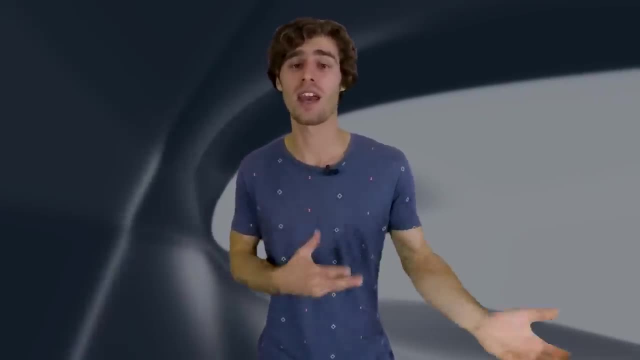 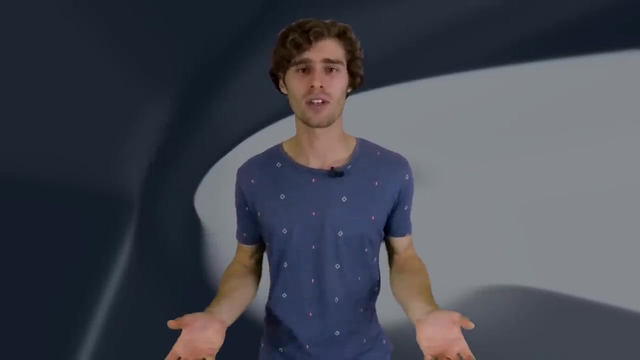 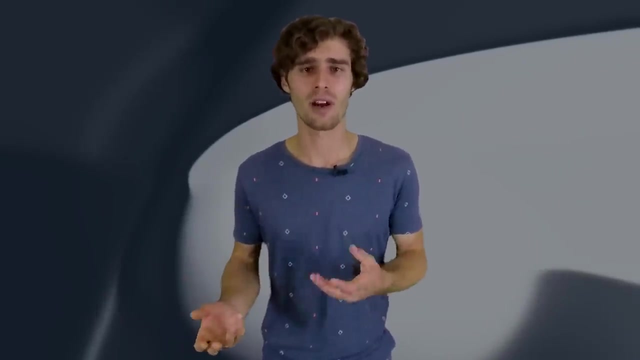 so, even though the value and policy outputs form two separate heads of the same network because they are part of the same computation graph, you can actually combine everything in a single loss function and the auto differentiation library will just figure out where to send all the gradients and the reason that these two loss terms are actually part of the same objective function. 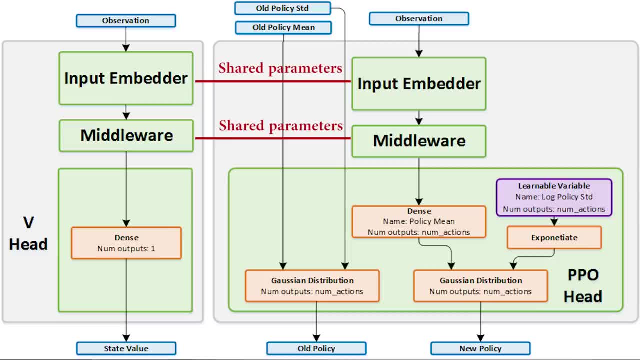 is that the value estimation network shares a large portion of its parameter space with the policy network, and the intuition is that, whether you're trying to- you know- estimate the value of the current state or you simply want to take the best current action, well, you're likely going to. 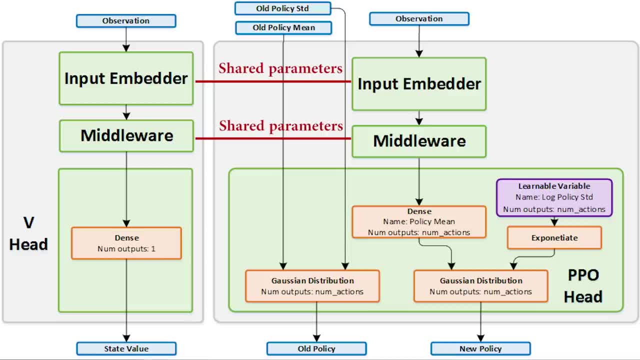 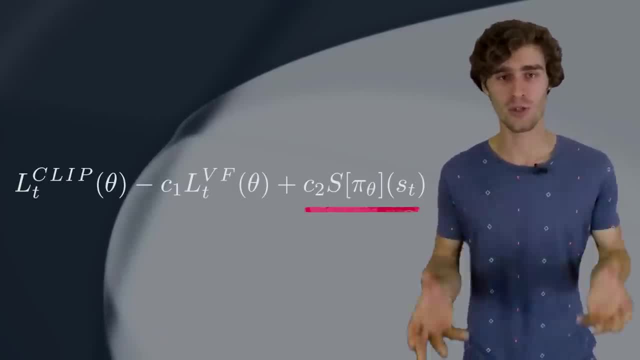 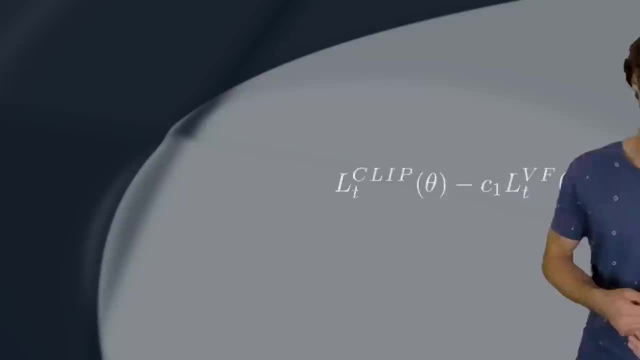 need very similar feature extraction pipelines from the current state observation, so these parts of the network are simply shared. and then, finally, the last term in the objective function is called the entropy term, and this term is in charge of making sure that our agent does enough exploration during training. so, in contrast to discrete action, 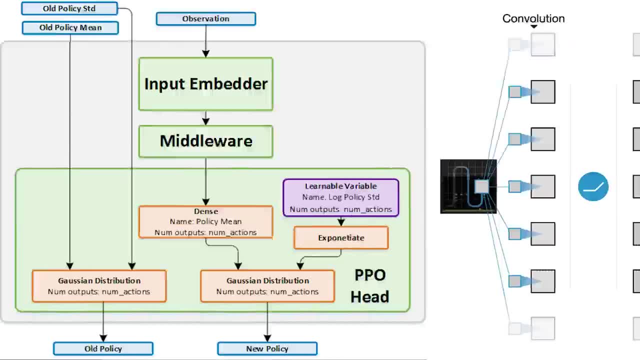 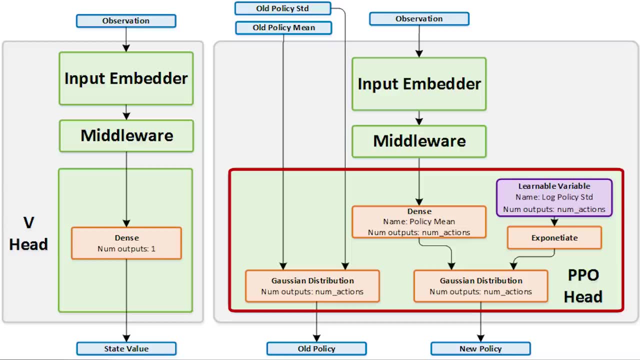 policies that output the action choice probabilities. the ppo policy head outputs the parameters of a Gaussian distribution for each available action type, and when running the agent in training mode, the policy will then sample from these distributions to get a continuous output value for each action head. now, if you want to fully understand why this entropy term encourages: 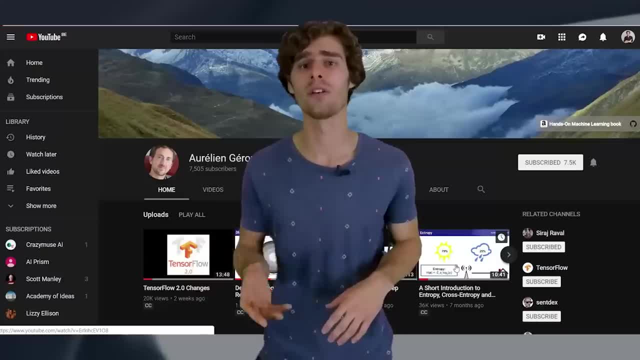 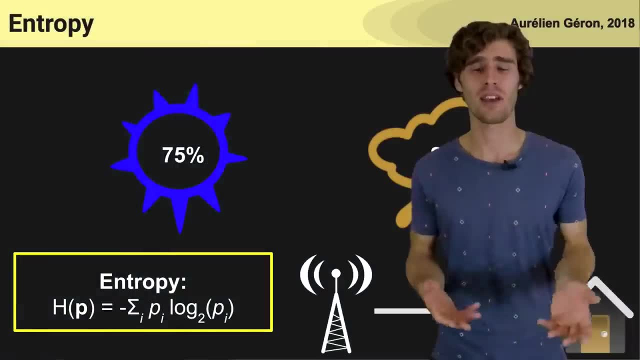 exploration. i really recommend to check out Aurélien Geron's video on the ideas behind entropy and KL divergence in machine learning. the link is in the description below. but basically, the entropy of a stochastic variable which is driven by an underlying probability distribution is the average amount of bits that is needed to represent its. 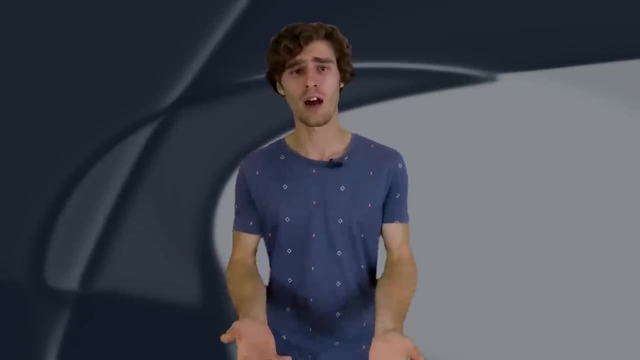 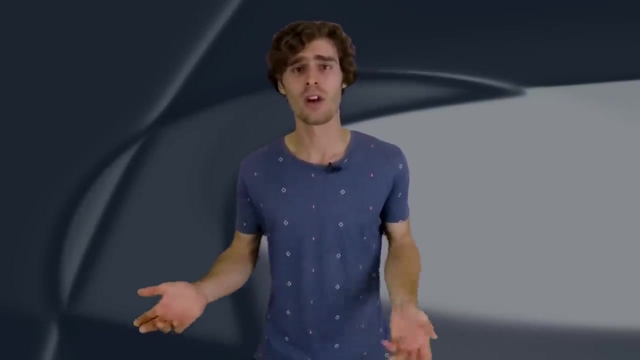 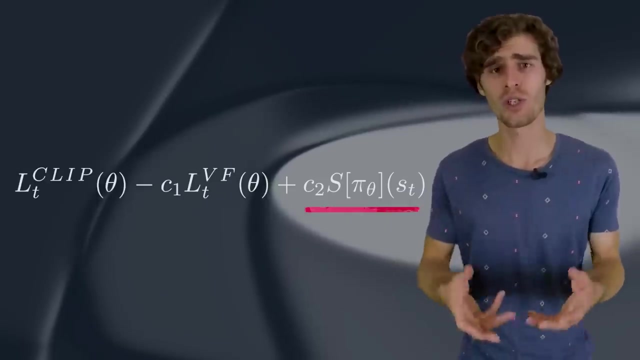 outcome. it is a measure of how unpredictable an outcome of this variable really is, and so maximizing its entropy will force it to have a wide spread over all the possible options resulting in the most unpredictable outcome, and so this gives some intuition as to why adding an entropy term will push the policy to behave a little bit more randomly. 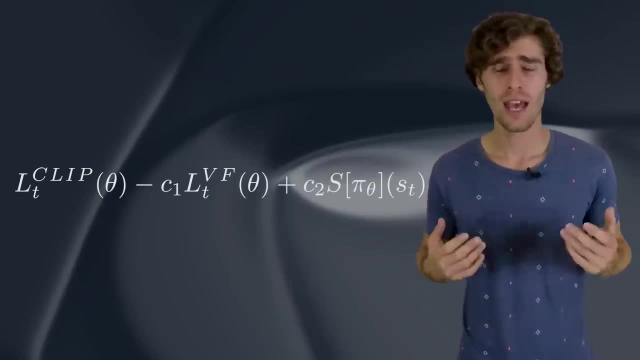 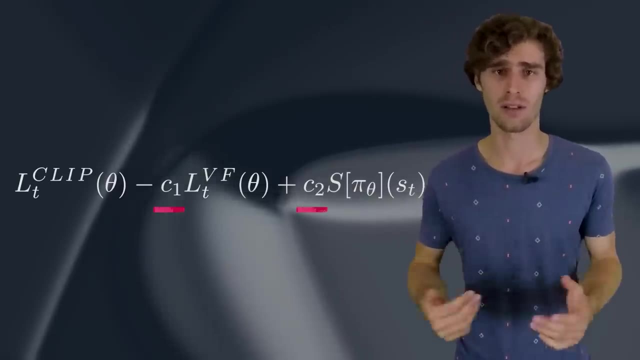 until the other parts of the objective start dominating and, as always, we have a couple of hyperparameters- c1 and c2, that weigh the contributions of these different parts in the loss function. now for people that want to take a deeper look at ppo in terms of python code: 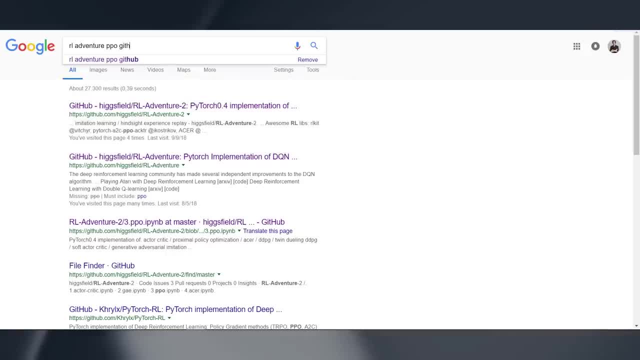 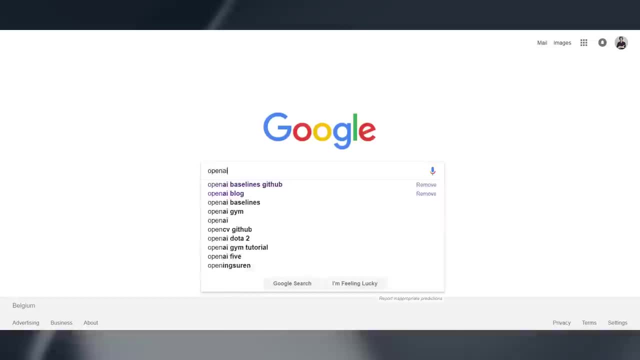 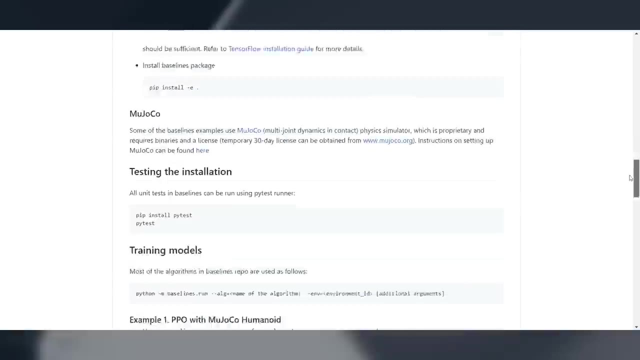 i really recommend to check out this implementation in pytorch from RLAdventure. trust me, even though you've never worked with pytorch, this implementation is as clean as it gets, and if you're looking for a more production proof implementation, i would recommend to check out openai baselines, which has a full implemented tensorflow version. 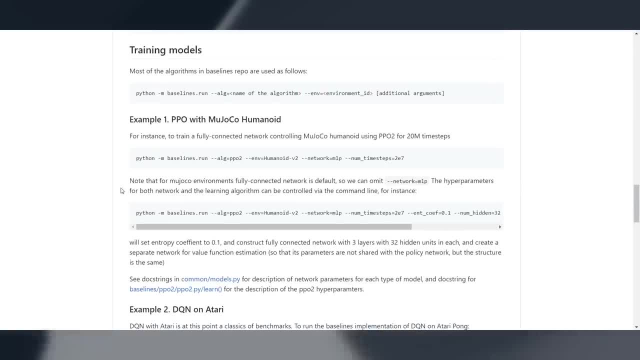 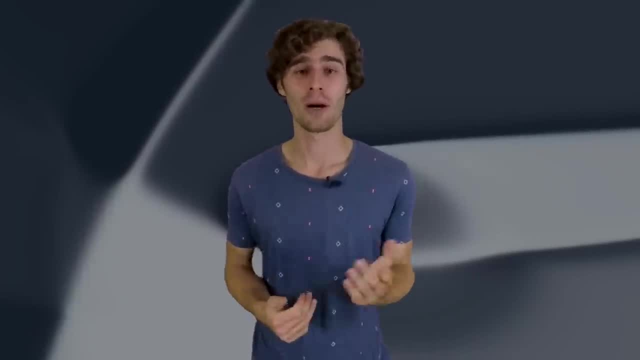 that runs on different environments, like atari, mojoco and others. both links are in the description. all right, so that's it. congratulations if you've made it this far. we've covered all you need to know about proximal policy optimization. now in the paper you can find a bunch of graphs that compare. 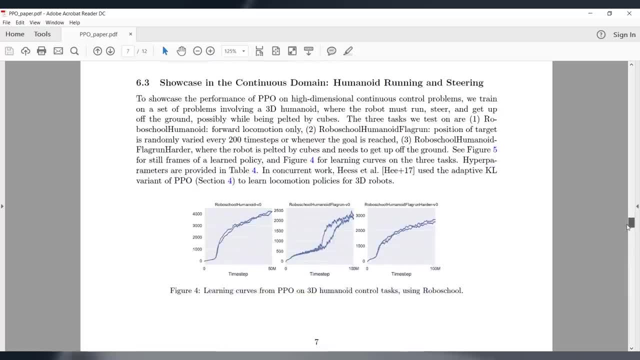 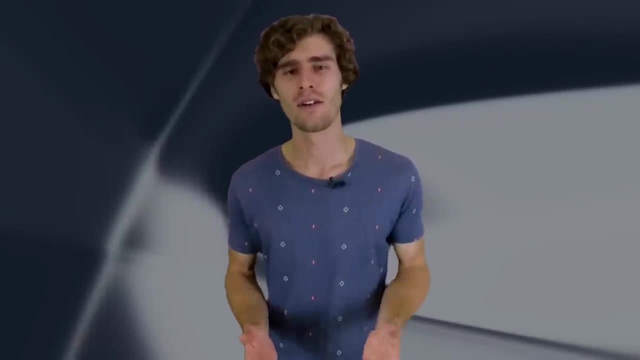 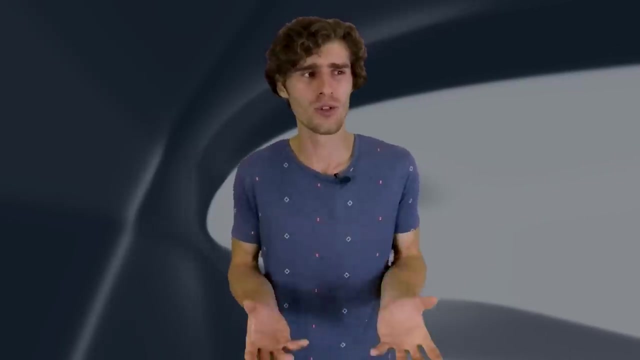 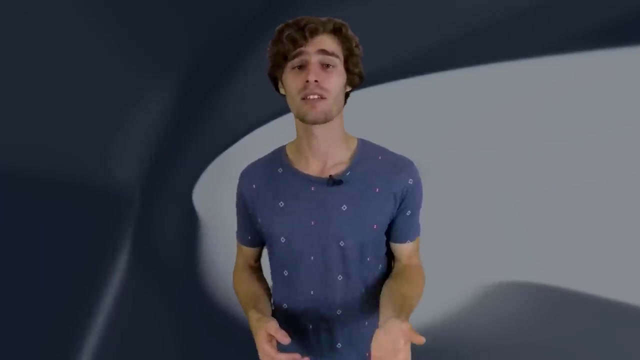 optimization of the ppo in the ppo and the ppo in the ppo, in the ppo, in the ppoоло ppoo, and that ppo was actually very, very complicated. it's one thing to remember, though, is that ppo wasn't specifically designed for sample efficiency, but rather to address the 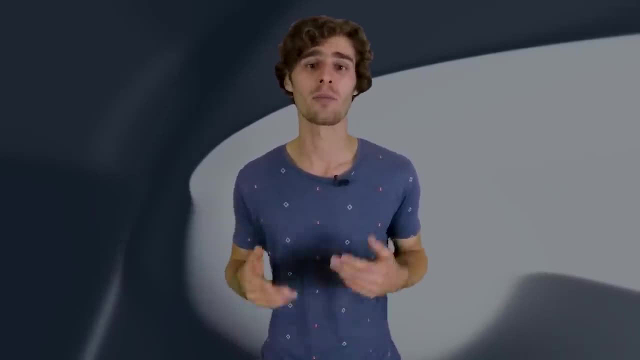 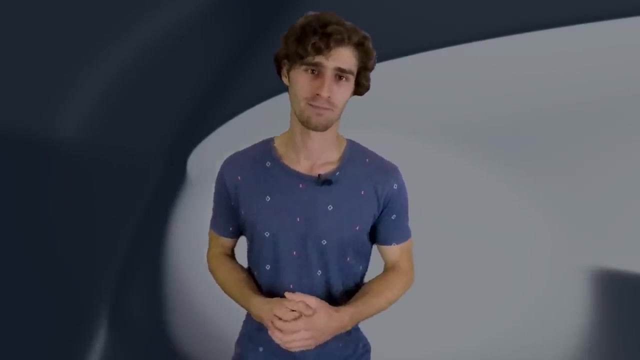 really complicated code that was needed for a lot of other algorithms and also, you know, making it relatively easy to tune in terms of hyper parameters, and because ppo achieves both of those objectives while also yielding close to or above state-of-the-art performance on a wide range of 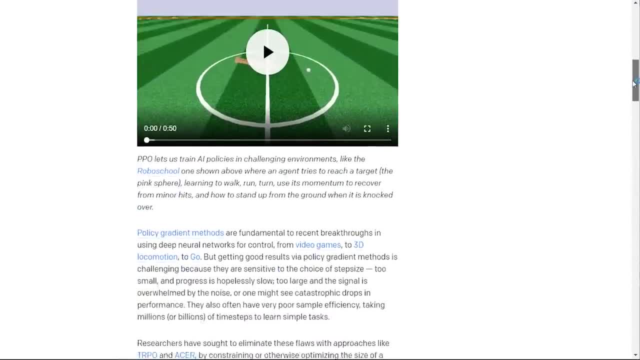 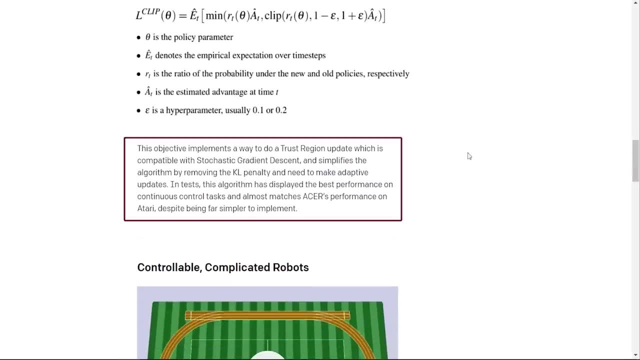 tasks. it has become one of the benchmarks in deep reinforcement learning. so, in summary, ppo is a state-of-the-art policy gradient method. the algorithm has the stability and reliability of TRPO, while being much simpler to implement, requiring only a few tweaks to vanilla policy.